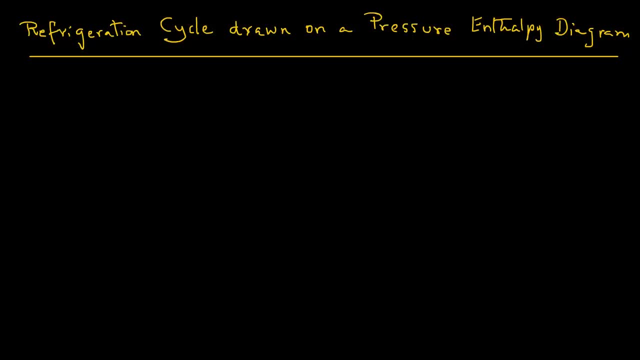 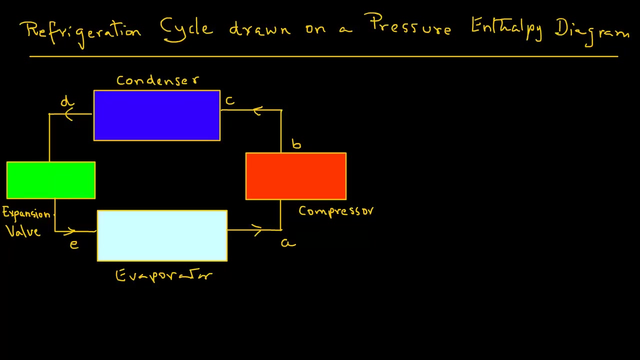 To get a better understanding of the condition of the refrigerant as it moves through various components of the refrigeration system, let us look at a schematic diagram and also a pH diagram side by side. So we will first draw a schematic of the refrigeration system. As you know, we have four components: compressor, condenser, expansion valve and evaporator. and recall the letters E, A, B, C, D that refer to the conditions of the refrigerant as it moves through the system. 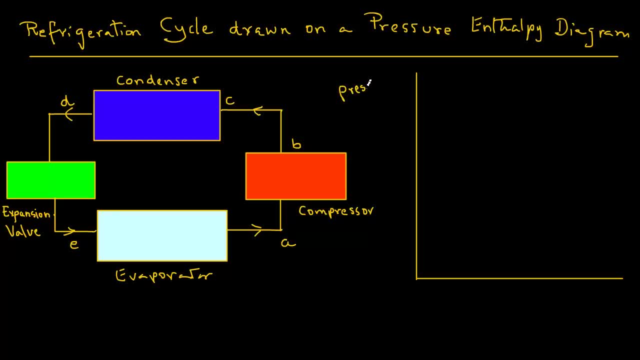 So now let's draw a pH diagram. We have the x-axis and the y-axis. Remember that pressure is shown on the y-axis and enthalpy is shown on the x-axis. We draw a bell-shaped curve, again skewed to the right, and now we will draw an ideal refrigeration cycle on this diagram. 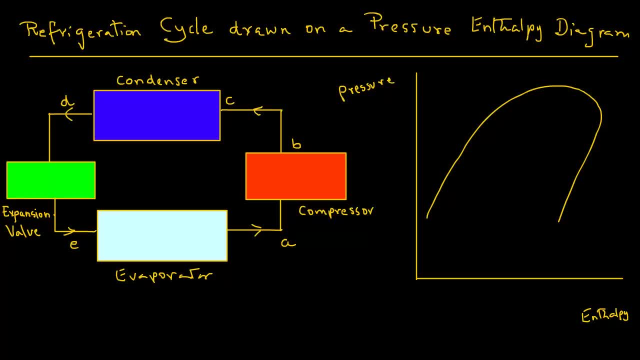 We will first draw a horizontal line originating somewhere within this region, going all the way to the right-hand side until it intersects The saturated vapor curve, intersects the saturated vapor curve And then from that point we will draw a constant entropy curve, skewed to the right, and draw a horizontal line on the top until it meets the saturated liquid curve and then drop a vertical line. 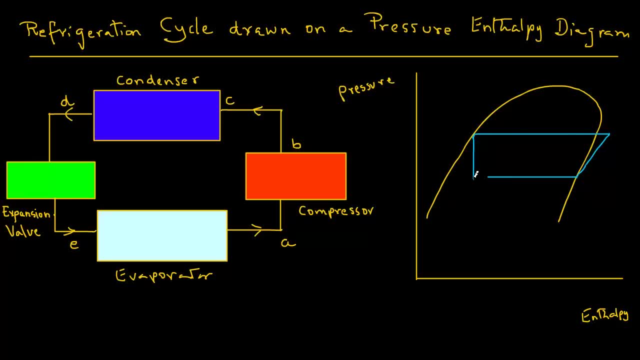 If it doesn't meet the horizontal line, we will just extend the horizontal line to make sure that it meets this vertical line, And so we have the ideal refrigeration cycle. And we will write down the letters E, A, B, C and D. 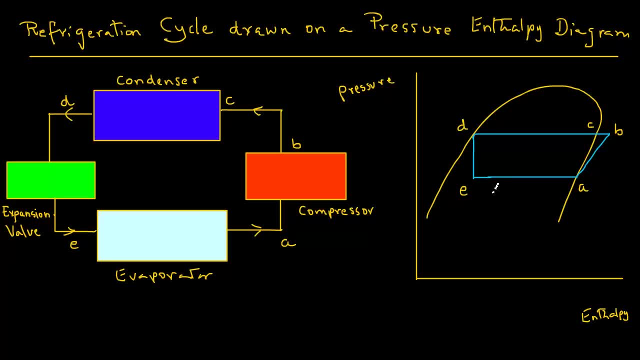 Note that from E to A we have the evaporator, As you know, as you can see on the schematic. so the same thing in this pressure enthalpy diagram. this is for the evaporator section. Part A to B is for the compressor And the horizontal. 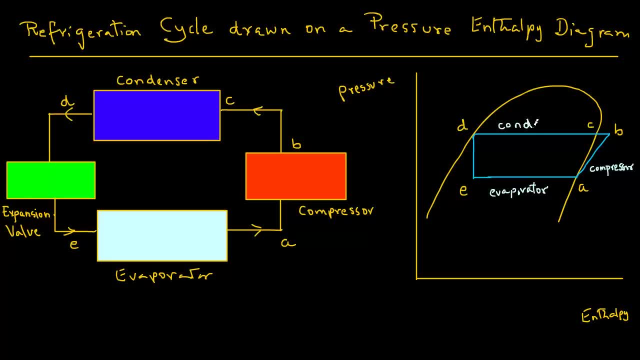 line on the top from B to D represents the condenser, And from D to E we have the expansion valve, And you can, of course, see these different components also shown on the left-hand side. schematic Note that the refrigerant is moving from E to A, A to B. 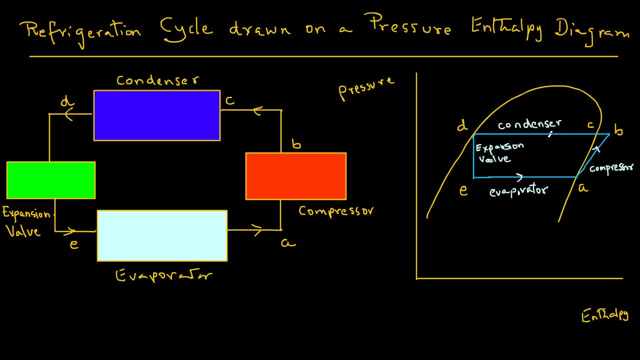 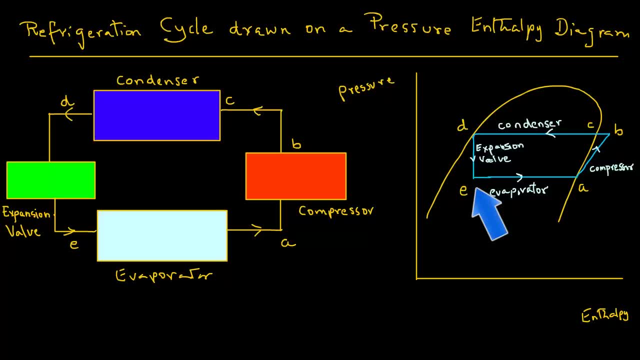 point is within this bell-shaped curve, and this region represents a mixture of liquid and vapor, So the state of the refrigerant is a mixture of liquid and vapor at location E. As the refrigerant moves through the evaporator, it absorbs here And then it moves through the evaporator And then it moves through. 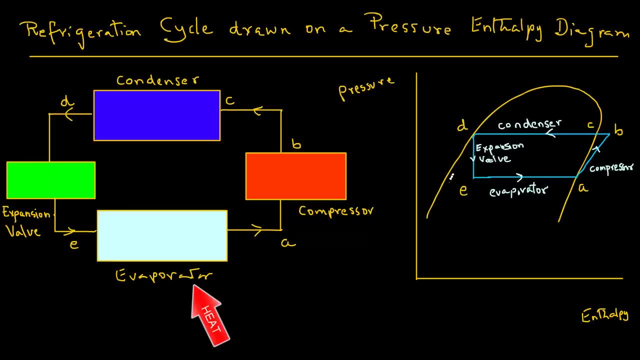 the evaporator And then it moves through the evaporator And then it moves through the heat from the surrounding and all the liquid turns into vapor. So by the time the refrigerant exits the evaporator, as shown by point A, the condition of the refrigerant is in saturated 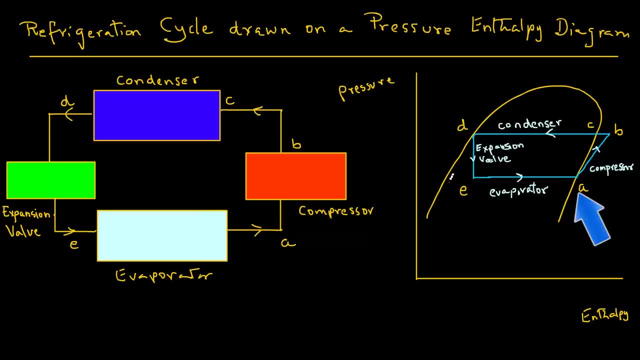 vapor state identified by point A being on the saturated vapor curve. Now in the compressor, the pressure is raised. So you see the increase in pressure And this is going from A to B. And as we note from thermodynamics that when you take a vapor, 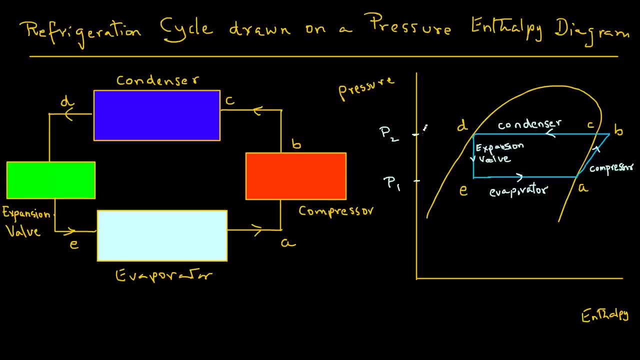 and you compress it. that process is isentropic. In other words, it's a constant entropy process. That is why we must follow a constant entropy curve in this region. At the exit of the compressor, the vapors are in superheated state. That's why this point. 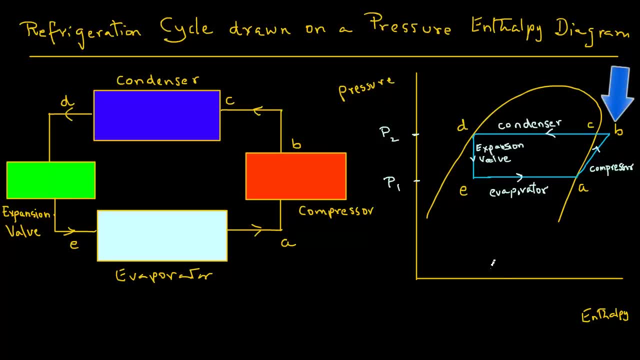 B is in the superheated vapor region. Now, from point B to C, as the refrigerant vapors exit the compressor, you first remove the superheat. So typically that part of the refrigeration system is called a desuperheater, although it is not shown here in the schematic. But most of the heat 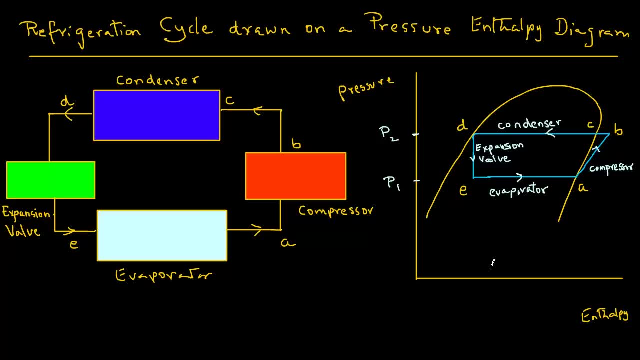 from the refrigerant is in the superheated vapor region And that's why we need to remove the superheated vapor region from here. And the especially important part for us at the exit of the compressor is to themselves remove the superheated vapor region from the compressor. 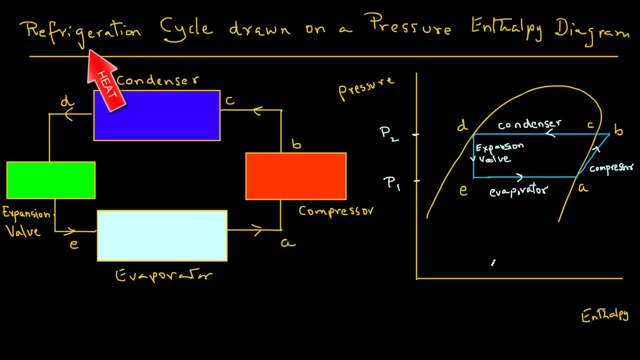 Because what we want to do is to remove the superheated vapor ever from the compressor, to remove the superheated vapor region, And that is, we need to remove the superheated vapor at least 5% of the vapor. Smokes will prefer the straight back towards the new capacitor. 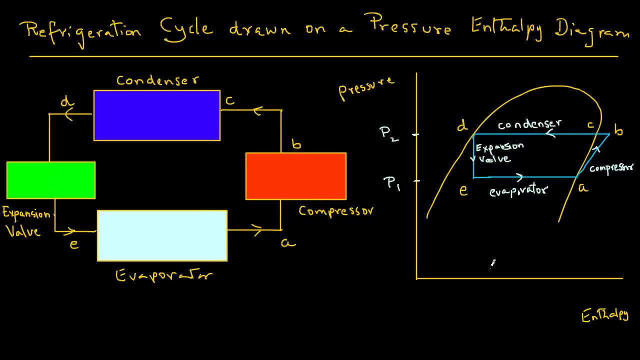 Because when the voltage rises you'll take off the ultraheated vapor and the інiceps returned is going to be a different distributor than Patel. So you know that you have a complex equation there. It's going to be問X, two STATES, Aerobic urine vacancy with ait become a total Creating Center for fizzy water flow. 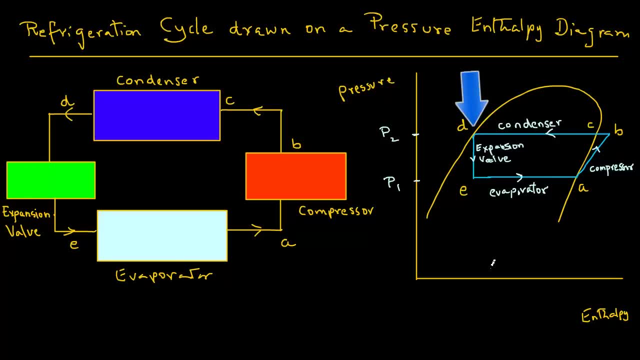 That's why this point is on the saturated liquid curve. Now, from point D, which is at high pressure, that high pressure liquid then enters the expansion valve, so there is a drop in pressure, So pressure decreases due to the expansion process and that process, again according to thermodynamics, is an adiabatic process. 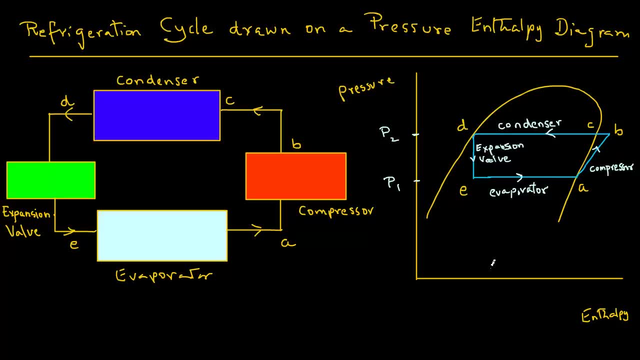 Recall that adiabatic means that the enthalpy remains constant. That is why we have a vertical line D to E, because that represents that the enthalpy, as you know from the x-axis, the enthalpy remains constant in the expansion process. 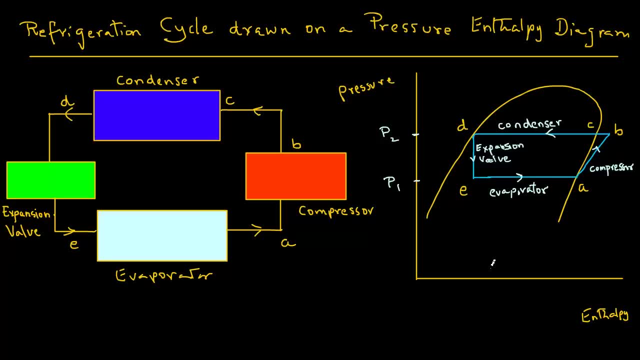 So at point E, then, as it leaves the expansion valve, some of the refrigerant is in vapor state but it's not in vapor state. So at point E then, as it leaves the expansion valve, some of the refrigerant is in vapor state but it's not in vapor state. 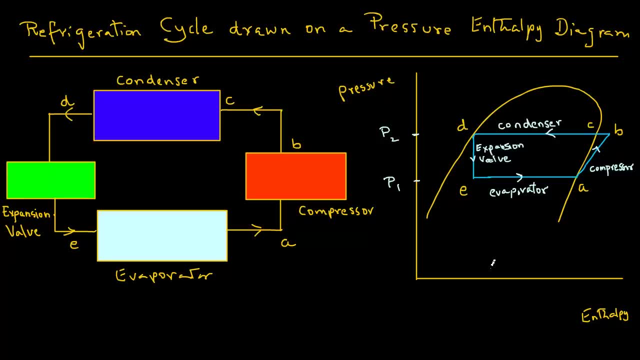 But most of it is in liquid state. So that point E represents a mixture of largely liquid but some vapors in the refrigerant that then enter the evaporator. So this is how the cycle continues. So note that in the evaporator heat is absorbed from the surroundings and in the condenser heat is discharged to the surroundings. 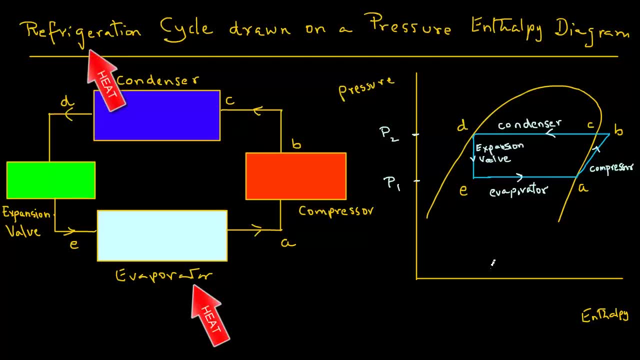 So this is how a refrigerant, A refrigeration system, can extract heat from one location and discharge it in another location. If you look at a refrigerator where the evaporator is located inside the refrigerator, it absorbs heat from the inside of the refrigerator, so all your food is cooled.